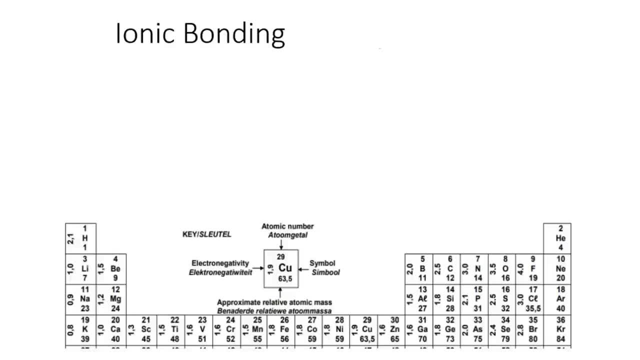 In this lesson we are going to look at ionic bonding. So ionic bonding is a type of bonding that takes place between metals and non-metals. So let's choose a metal. Let's choose lithium, for example. So we know that I want to just quickly go draw the whole structure, but eventually we'll. 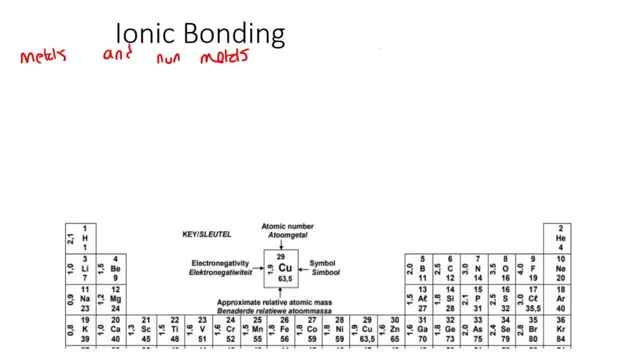 only be using the Lewis diagrams. But if we just draw the structure of lithium, we know that it is. it has a positive protons, or it's got positive protons in the middle, or positive nucleus. that's what I was going to say. Then it's in row number two, so it's got two energy levels on the outside. 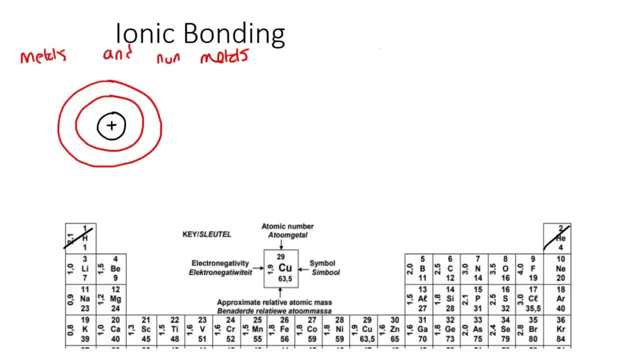 and so in energy level number one it's going to have two electrons, and then in energy level number two, it's got one electron, so it looks something like that. Okay, now I want us to look at chlorine. so it has a nucleus which is positive, and then it's an energy level number three, so it's going to have three energy levels. 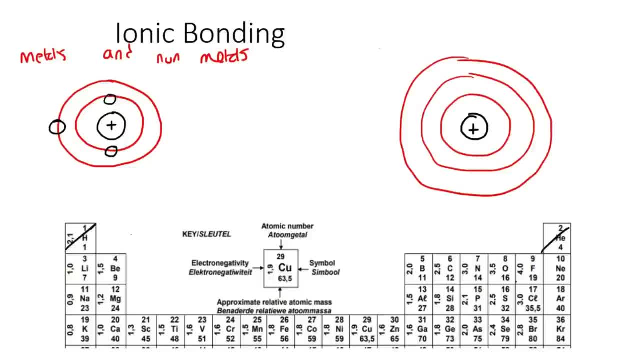 In energy level number one, it's going to have one, two electrons. In energy level number two, it's going to have one, two, three, four, five, six, seven, eight electrons. and then, in energy level number three, it's going to have one, two, three, four, five, six, seven electrons. one, two, three, four, five. 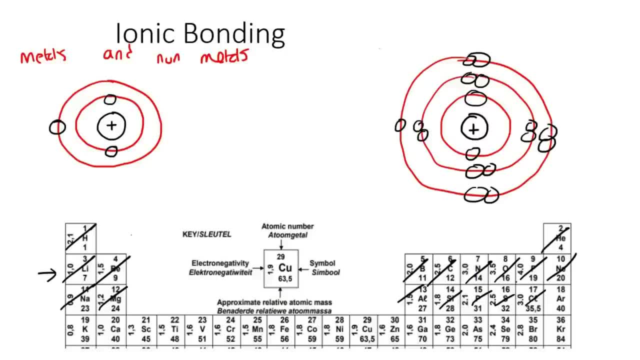 six, seven Now, in a previous lesson. well, let's just first say that this is lithium and this is chlorine. in a previous lesson we learned that the main reason that atoms bond, atoms bond in order to have complete outer energy levels. And in that lesson we learned that, for example, lithium over here would give, would rather lose. it would give this electron away. 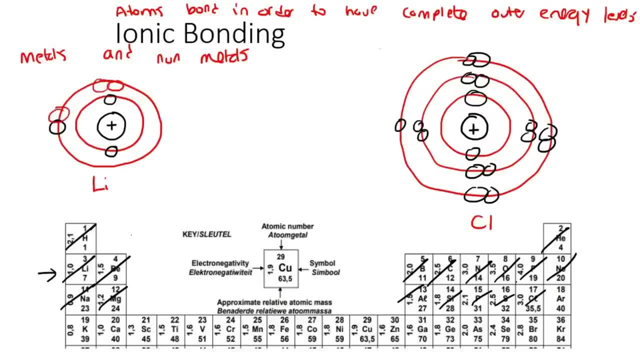 because it would be more difficult for it to try gain seven electrons. It won't do that, It would rather give this electron away. And what we learned was that this chlorine already has two, four, six, seven electrons on the outside. It only needs one more to have eight, which is a complete energy level. 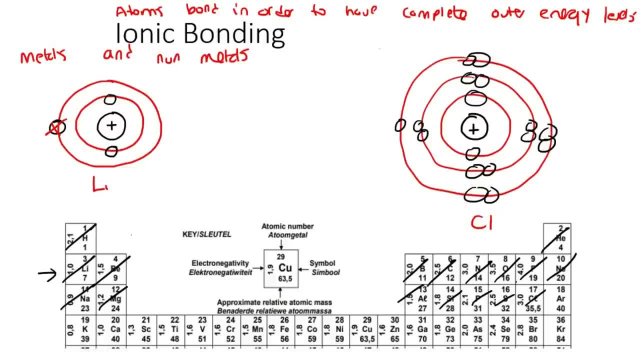 So all that happens when these two bond is that this lithium is going to lose its electron. It's going to give its electron away, okay, And then that electron is now going to be floating over here And that electron is simply going to go to this. 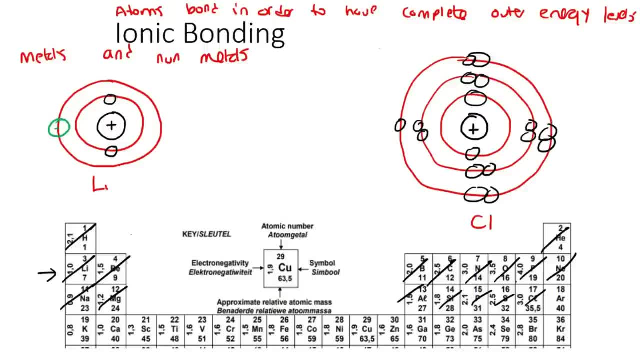 Well, let's actually do something like this: Let's put a little green one over here And that's an electron, And then what happens is that this green one is going to be eliminated, or it's going to be removed from there And it's rather going to go and land up over there. 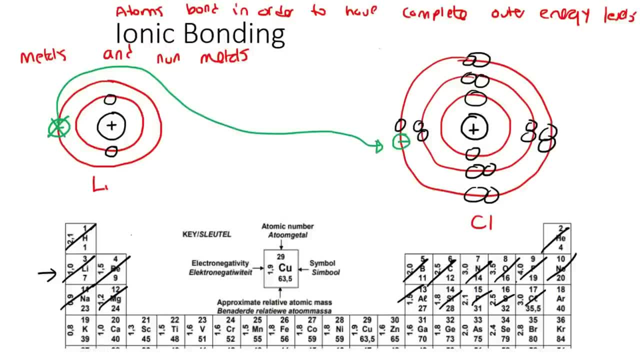 And what happens now is that this lithium is now very happy. Why? Because it's still got a nucleus, but now the outer energy level, this energy level, we can take that one away. So we only have one outer energy level now and it's complete because, remember, energy level number. energy level number one, or row one, only has two places that need to be filled. 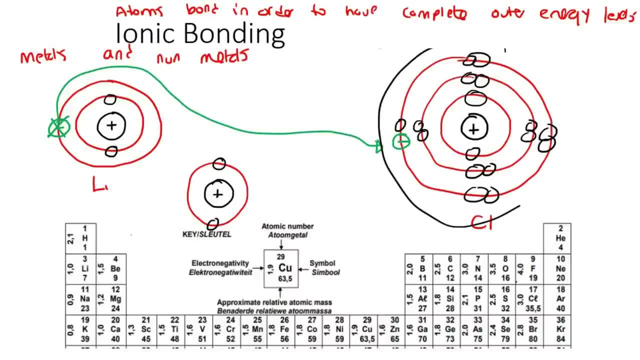 So this is now complete. Now this chlorine is very happy because, look at this, It's got two, four, six, eight, So it's got a complete outside energy level. So both atoms are very happy now because they both have complete outer energy levels. 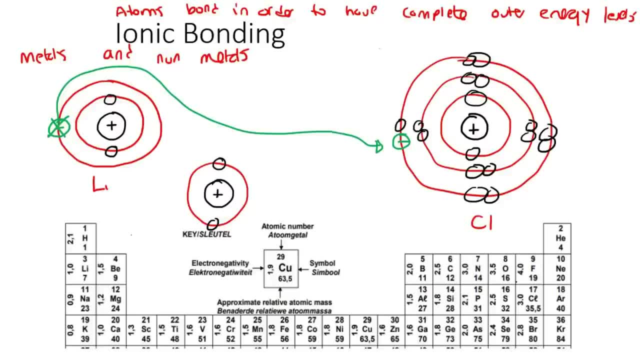 So can we see what happened? That the metal, which was lithium, gave its electron to the nonmetal. So that's another thing about ionic bonding: The metal gives electron, or electrons, to the nonmetal. OK, that is ionic bonding. 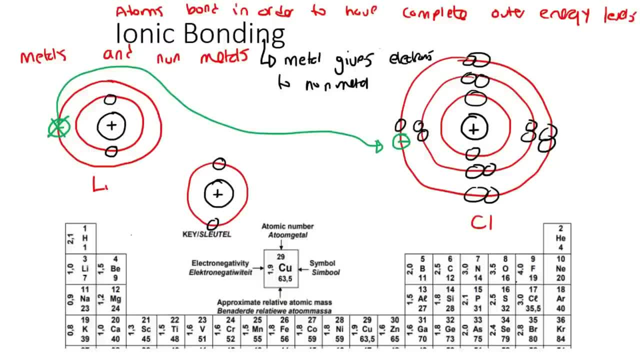 It's when a metal and a nonmetal- the one gives its electrons away and the other one accepts it. Now the next thing we need to talk about is what is going to happen to this atom now. Is it going to become positive or negative? 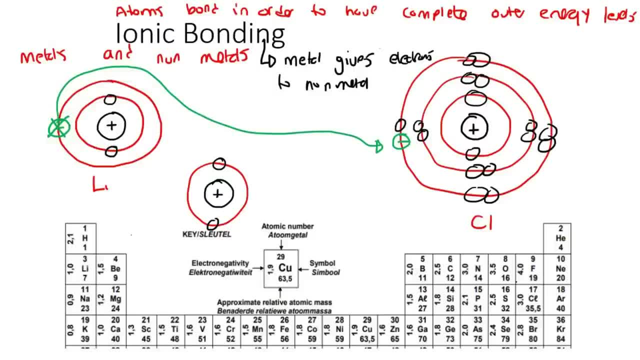 Well, over here it had three protons, because it's over there, and it also had three electrons which are negative. That's what it had over here. But then over here it's still going to have three protons, But it only has two electrons. 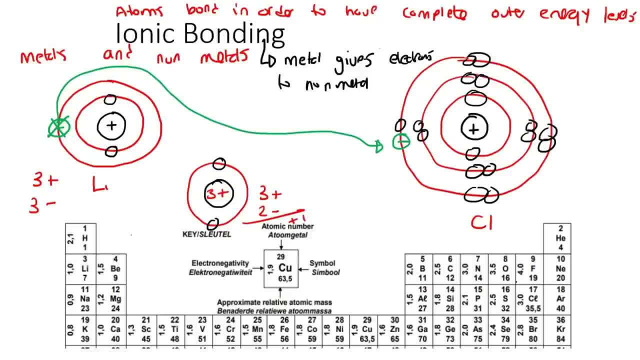 And so, if you had to add that up, it's now going to be positive. So this, this atom, is now going to be positively charged. If you had to go and look at this atom over here, you would see that because it gained one electron, it's going to be negatively charged. 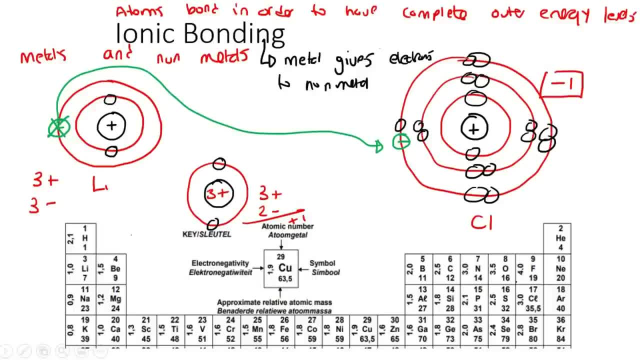 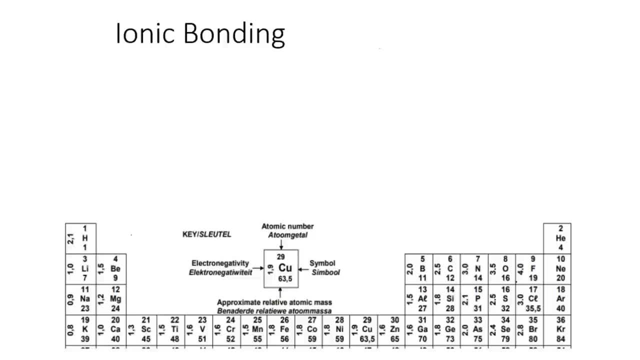 It's going to have a negative one charge. OK, so the way that we're going to do this from now on Is we are going to show ionic bonding by using Lewis Diagrams. So if we go and draw lithium, We know that lithium is in group one. 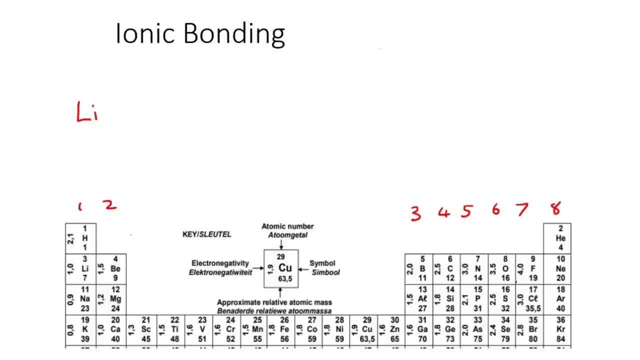 OK, remember Lewis diagrams. you only need to know the groups. So lithium is in group one, So it means it's got one valence electron. OK, we only going to show the valence electrons. We're not going to show, we're not going to show all of the. 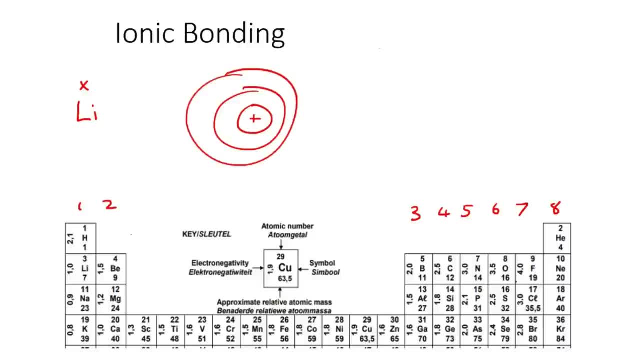 So, for example, if that's lithium, we're not going to go show all of the electrons, We're just going to show the valence electron part, Which is the Part that's on the outside, And that's what the Lewis diagram does. 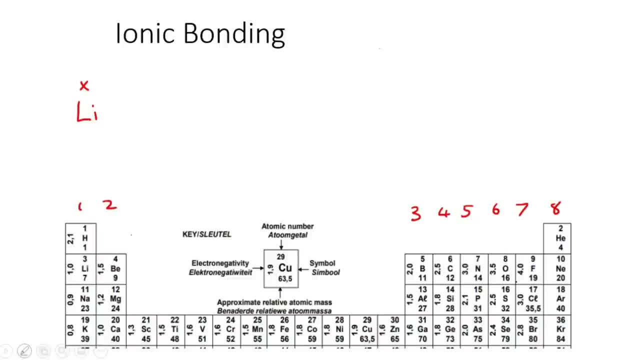 We know that it's got electrons on the inside, but we're just showing the valence ones. OK, and now what we're going to do is we're going to go show chlorine. So chlorine is in here in group seven. So that means it's got seven valence electrons. 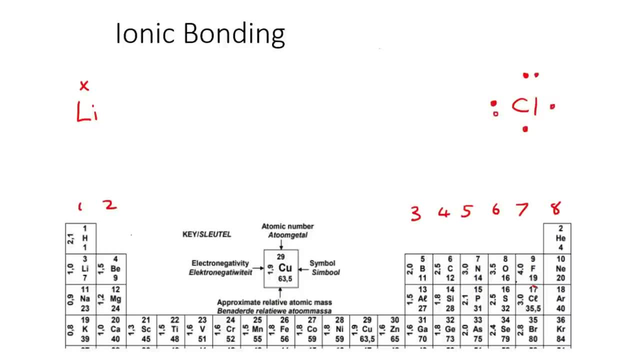 So one, two, three, four, five, six, seven. OK, now, what we learned a few moments ago was that this electron here, I mean this atom, is going to lose this electron. So what we're going to do is we're going to say that this gets converted into a lithium, which is now going to be positively charged. 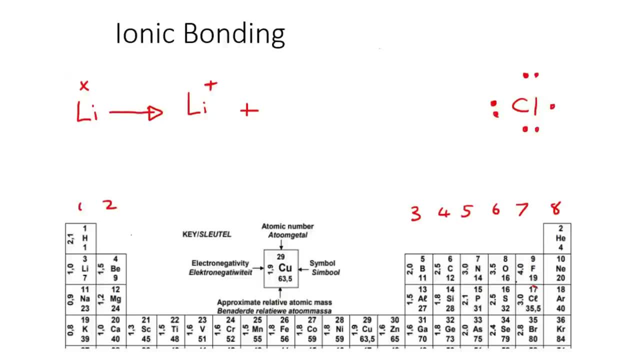 And then it's going to give away this electron over here. OK, so you could. you could write your electron. So let me just explain this part carefully, because learners get a bit confused here. What happens is that this lithium, which has one electron, on the outside, it's got one valence electron. 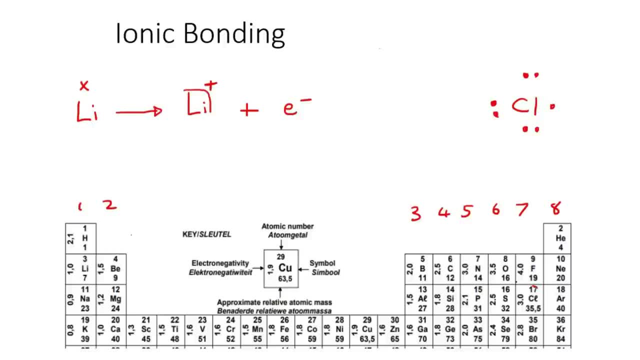 When it gives that electron away, then it's going to become A lithium with no electrons on the outside. You see, there's no electrons on the outside. It's been given away. And because it gave an electron away, it becomes positively charged. 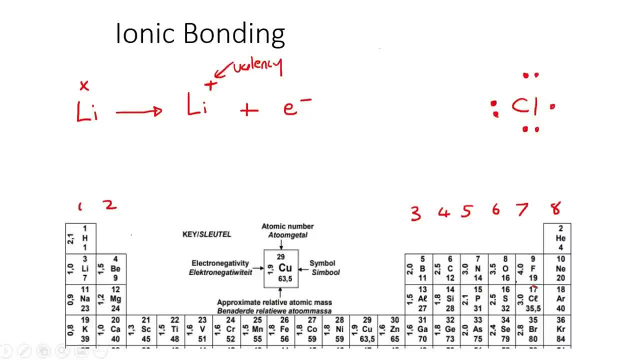 OK, that's like it's valency, This is its valency, OK, and then it also gave away. So so, so then it also gave away this electron over here. So let me try to draw that nicely for you. We had a lithium atom which had one electron on the outside. 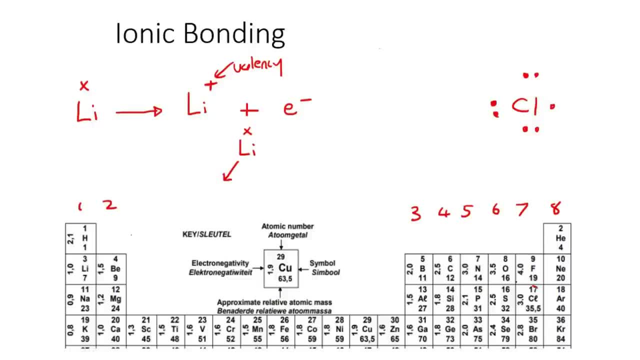 One Valence electron, And then we converted it into a lithium with no electron on the outside. So now it's positively charged And then it also that that electron that it gave away is now over here floating around in the atmosphere. OK, what happens with the chlorine? 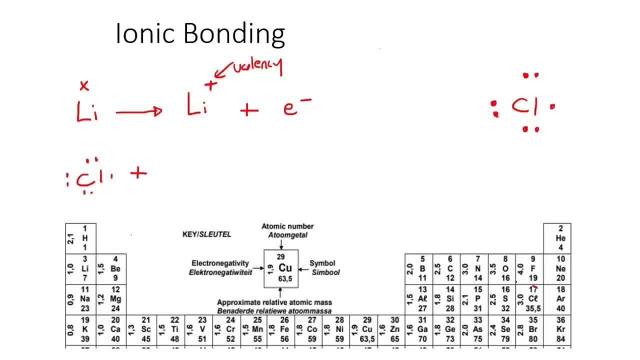 Is that the chlorine is going to add with this electron, So it's going to combine with this electron and together it's going to become chlorine, like this With the X. you see, So what's happened is that this X has landed up going over there, but this is the way you would show it. 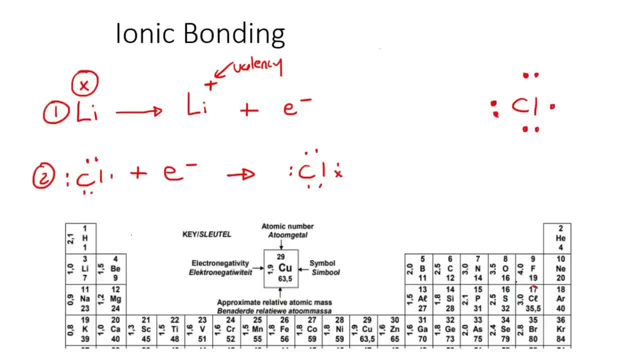 This is step one. This is step two. Now, what's important is that this chlorine is now negatively charged because it got one electron, But when there's a whole bunch of things around it, you must just put it in a square bracket like this, and you're going to put a negative one like that. 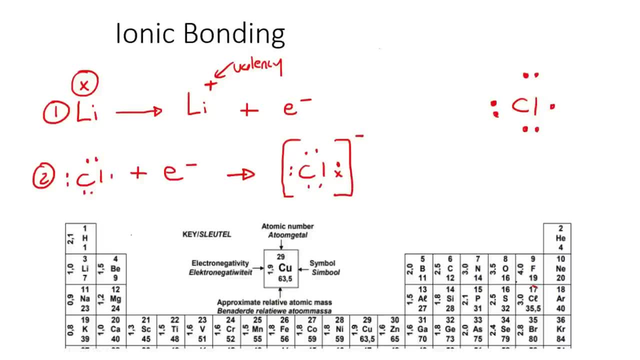 Or you could actually just put a negative like that. Now, the third step Is that this lithium is now positive and this chlorine is now negative, so they are going to be attracted to each other. so we can say that the lithium which is now positive is going to attract to the chlorine which is now negative, and they are going to be converted into a structure that looks like this: 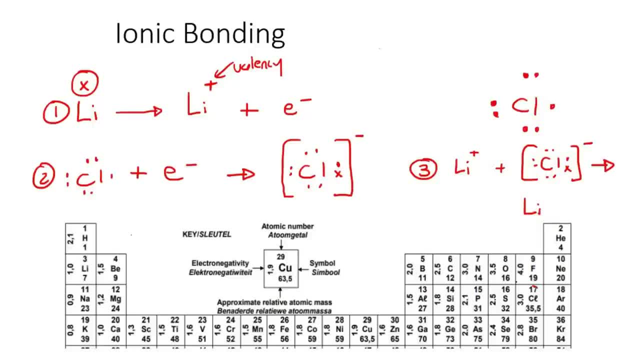 You're just going to put them next to each other. So you're just going to put them next to each other with its little plus, and then the C, Now with all of its things, which is negative, and then your teacher might go one step further and just take away the plus and the minus and all the brackets and they'll just say L, I, C, L. 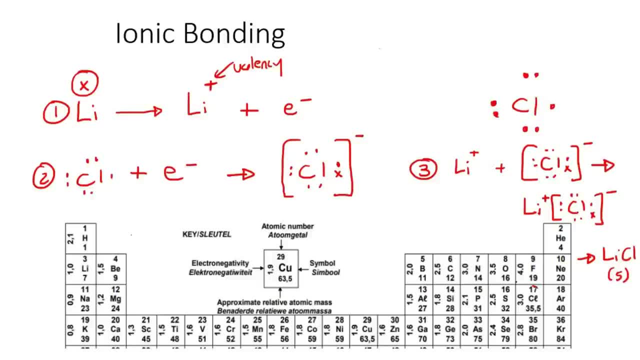 And then they might even say that that is in the solid phase. OK, so let's do a whole bunch more examples of ionic bonding now. I know that right now you might be feeling a little bit confused about what we've just done. 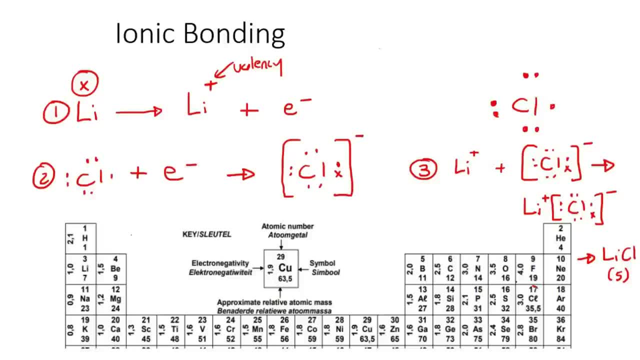 That's normal, But now let's do some more examples, And we have got quite a challenge. We have got quite a challenging example coming up at a later part of this video, so stick around with that It's going to. it's going to be involving weird numbers and things like that. 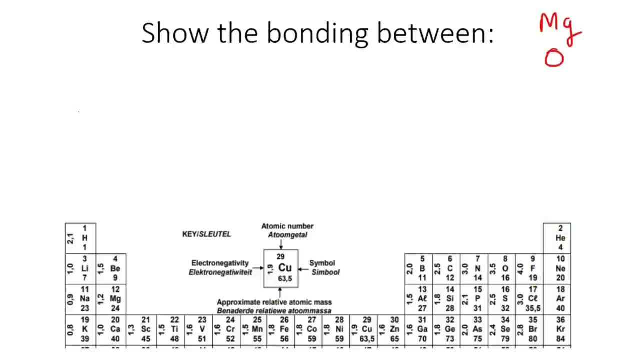 In this example we're going to look at the bonding between magnesium and oxygen. Step one: draw a Lewis diagram for each one. So we're going to look at because we need to try figure out: is this going to be ionic, covalent or metallic? 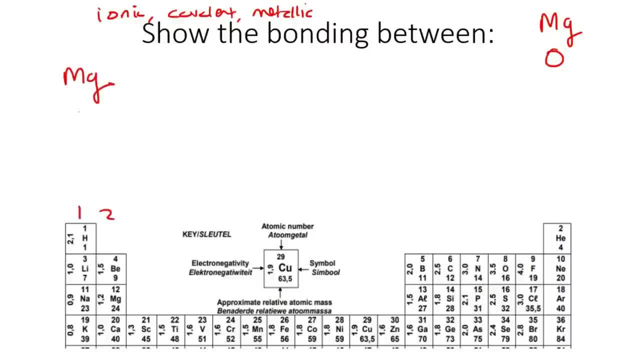 So we're going to go look at magnesium Now. magnesium is in group number three. It's got two on the periodic table There it is. So that means it has two electrons, two valence electrons. Obviously, it's got 12 electrons in total. 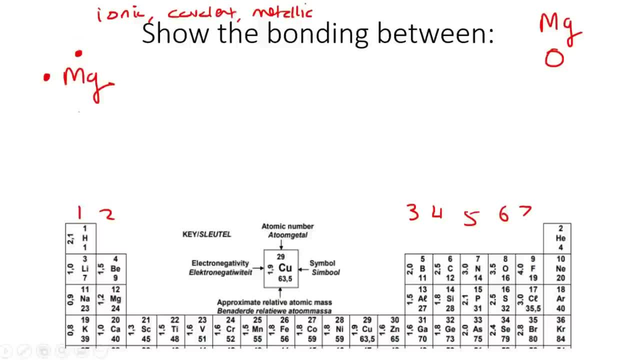 But for Lewis diagrams we're only looking at the electrons on the outside, the valence electrons. Now we're going to do oxygen, So oxygen is in group six. OK, so it's got six valence electrons. It's got eight electrons in total, but six of them are valence. 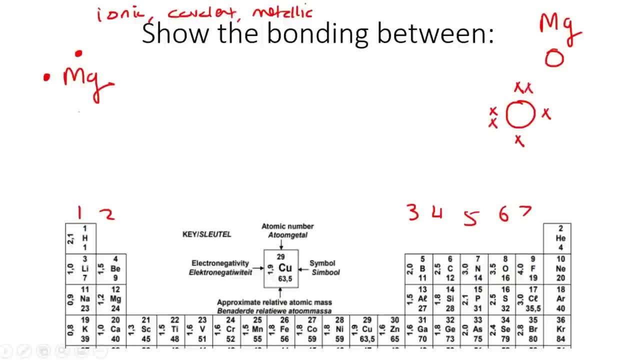 And once again we only look at valence. Now can you figure out a nice way to make both of these atoms happy? Well, would it be better for this one to lose all of those six electrons, Or would it rather be better to just gain two of them, two electrons over there. 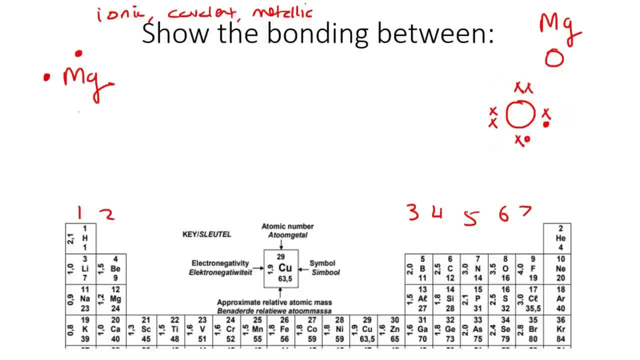 Because if it can gain two electrons, then it will be complete. The other thing is: would it be better for this one to try to gain six electrons so that it becomes complete, Or would it be better for this magnesium to simply gain? Or would it be better for this one to try to get rid of those two electrons, and then it will be complete as well? 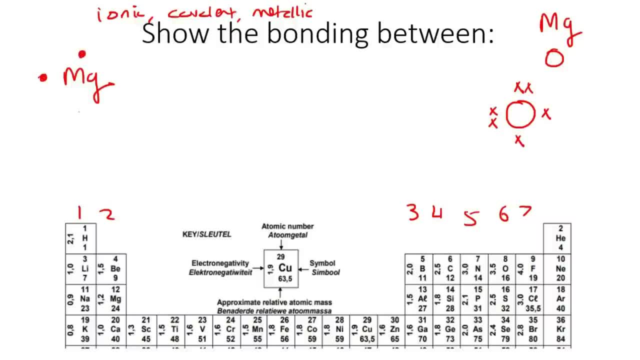 Well, if you've watched the previous lessons where we spoke about how the how different things gain electrons, different things lose electrons, you'd see that this is a metal and metals lose electrons. It'll be easier to lose these two electrons and it'll be easier for this one to gain those two electrons. 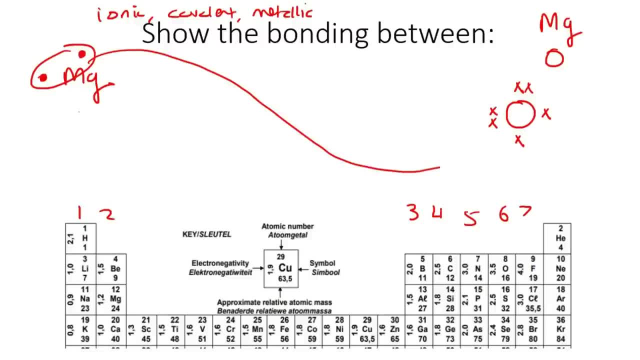 So what happens is that these two electrons are just going to be donated To this atom over here, And so your end result is going to look something like this: But we need to show how that all happens now. So step one: we're going to take this metal. 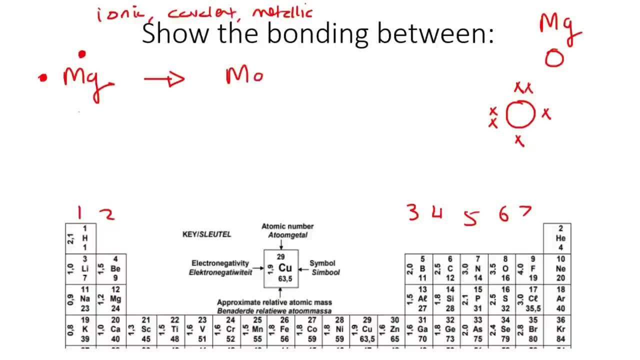 And we're going to show how that metal loses those electrons. So have a look here, Whoops. You see how it's got no more electrons on the outside, no more valence electrons. It lost them, And so we need to show that those two electrons are now over there. 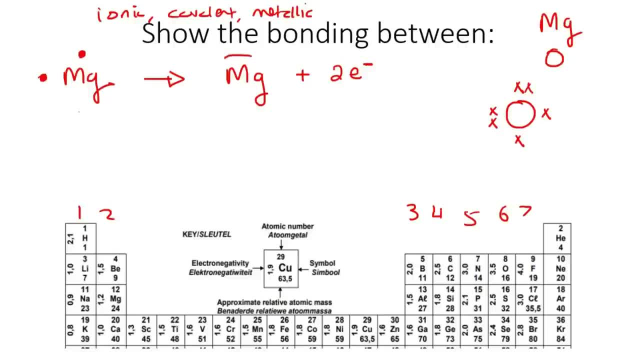 OK, that's step one. Oh, and then, and then what did? if this magnesium atom over here Loses two electrons, then it will become positive, and that's where valency comes into it. So it's valency is positive too. 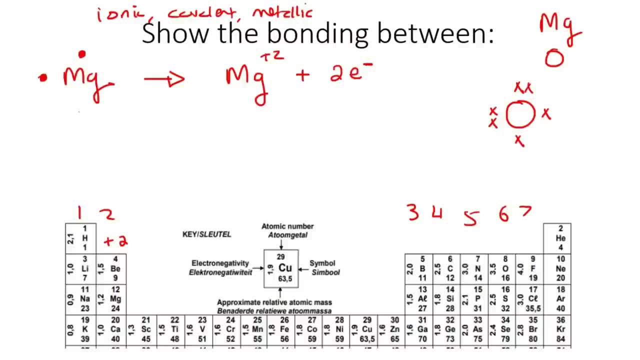 So it becomes positive. OK, now those, this, this oxygen atom is now going to add those electrons to it, And what will happen is that it will become like that, And because it now added two electrons to it, it becomes negatively charged. So you can do that. 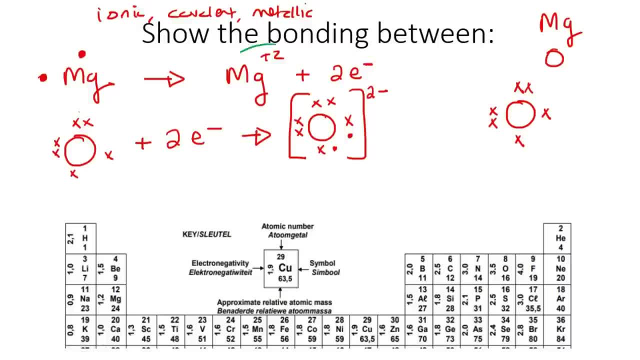 Now the third step Is to show that this positive ion- over here, by the way- this is an ion. An ion is a charged atom or molecule. OK, so this one is positively charged. We call that a cation, by the way. 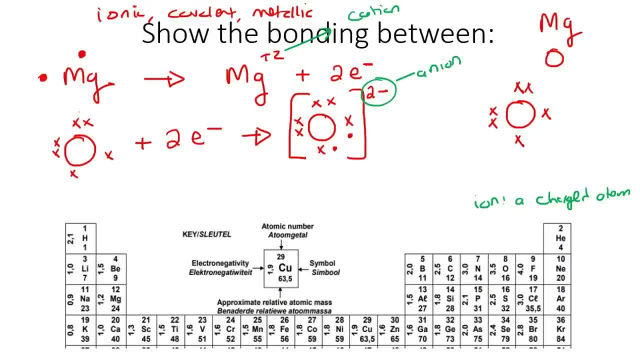 And this one is negatively charged. We call that an anion. OK, so what happens now is that those two ions are oppositely charged- This one's positive, This one's negative- So they are going to be Attracted to each other. 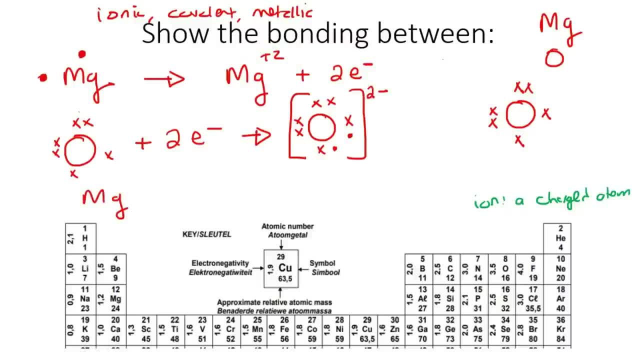 And so the last step: We have to go and put those all together. So we're going to say Mg plus two plus the oxygen part, And what happens is that that now just becomes. you're just going to write them next to each other. 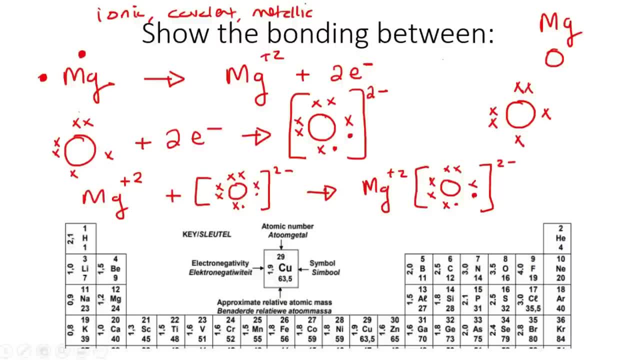 So Mg plus two with oxygen, two minus, And then your teacher might go one step further and just say that that will become MgO, which is a solid. Let's do another example. Now it's going to start getting a little bit more challenging. 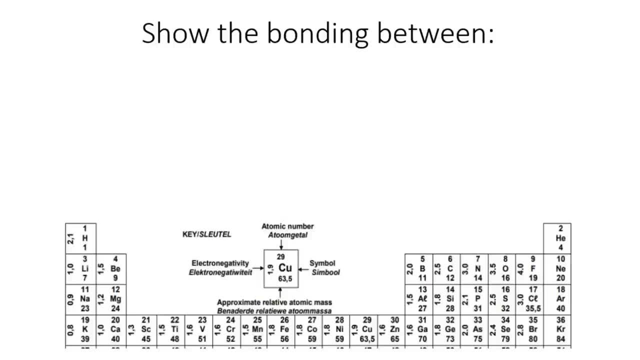 So let's not do an example between Lithium and oxygen. so step one, go draw the Lewis diagram. so the Lewis diagram only uses the valence electrons. so that's just by looking at the group number. So lithium is in group one. 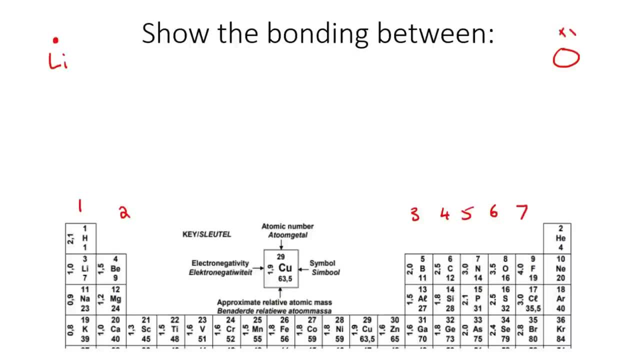 Oxygen is in group six, so that's going to be one, two Whoops. it's rather do it the proper way, You put one at a time And then you go again. There we go. Now we know that lithium is going to lose one electron. 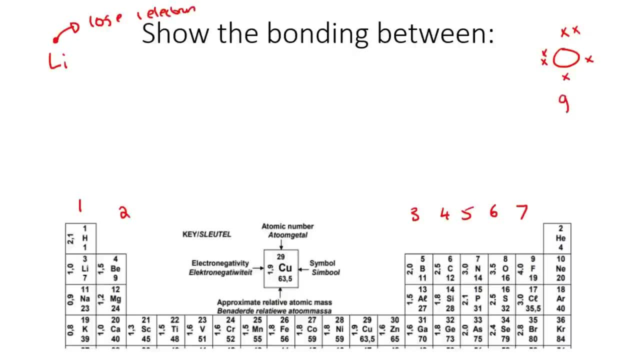 And then oxygen is going to gain two electrons. Why? Because then it will be complete. Okay, And remember, when I show you lithium, we must always remember that lithium actually has two energy levels: The. Oh wait, That doesn't look nice. 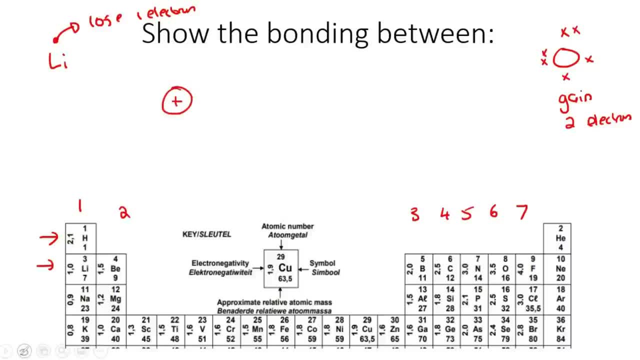 Let's do. It's got a positive nucleus and then it's got Two energy levels. Okay, And in energy level number one it's got two electrons And then an energy level number two it's got one electron, But we only show this one in a Lewis diagram. 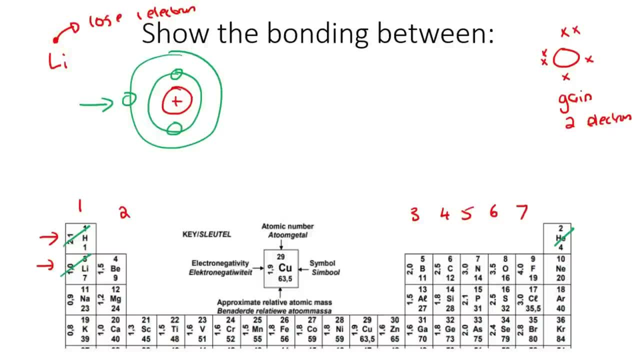 So when it loses that electron, It then has that, And so it would be fully complete. Okay, And that's stuff we've learned about before. So, and then this one is going to, rather gain, This one's going to try to gain- two electrons so that it can be complete. 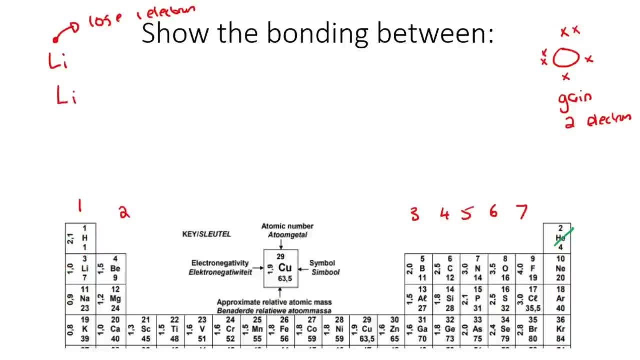 Okay, So let's show how lithium loses that electron. So you're going to say lithium, Let's do it here, because this, this example, is going to be a bit more interesting now. So lithium is going to be converted into a normal lithium ion with no valence electrons. 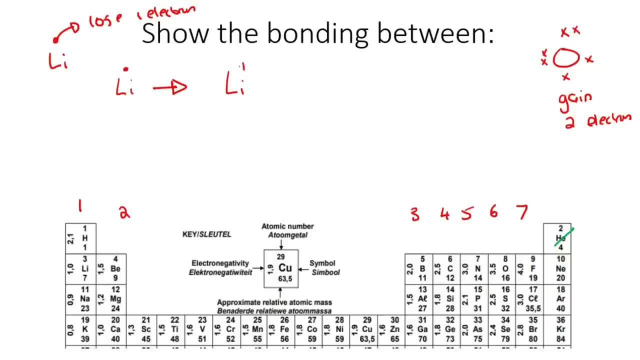 Okay, But because it's lost an electron, it becomes positive, And then the electron that it gave away is here Now: oxygen. Here's where things get weird. Oxygen needs two electrons. Okay, So oxygen needs two electrons in order to be able to fill up this entire energy. 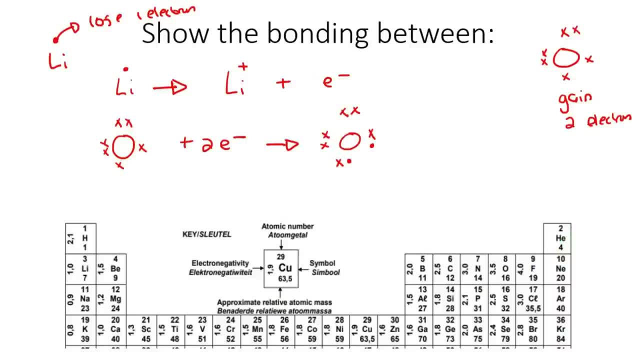 So it's going to go like this, And then, because this oxygen now has two extra electrons, it's going to become negatively charged. So we'll say negative two or two minus Okay, And that's the same as its valency, Okay. 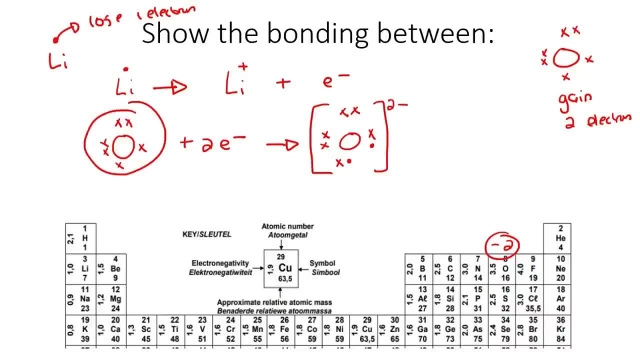 So what we have is that this oxygen over here needs two electrons, But this lithium only gave away one electron. So when this happens, we have a bit of a problem, because how is this oxygen supposed to get two electrons if this lithium only gives away one? 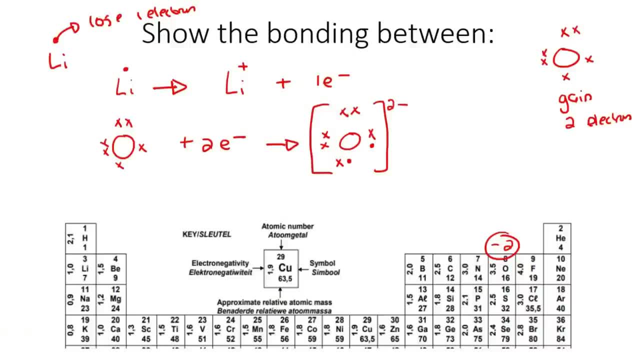 What you do when this happens is you have to make sure that these two numbers are the same. So we're going to multiply this entire reaction with two. Okay, So that means we're going to put a two in the front there, a two in the front there. 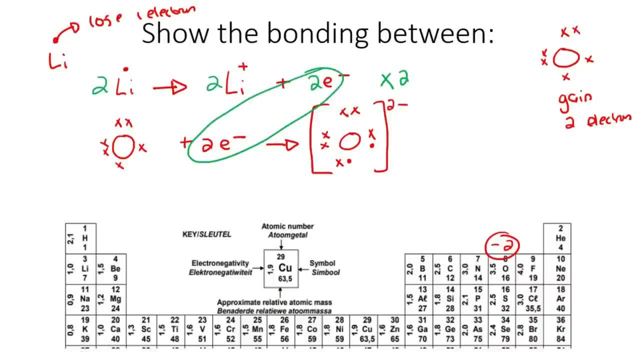 and this will become a two. Now, when these two are the same, you are going to combine them, like we normally do, So we're going to take the cation, which is the positive one. You're going to add it to the anion. 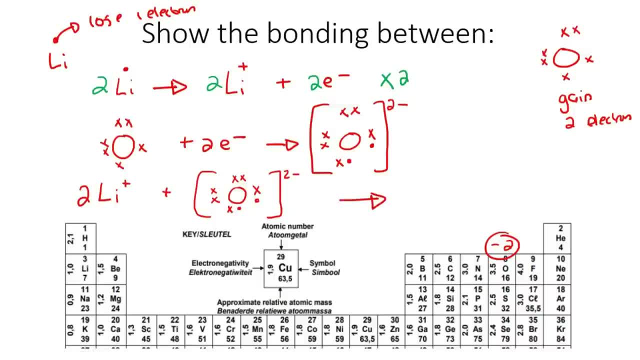 And what you then form is: you just put them next to each other, like this, like that. Now, your teacher might then write it in a different way, where they'll say: okay, so we have two Li's, So you'll say: Li. 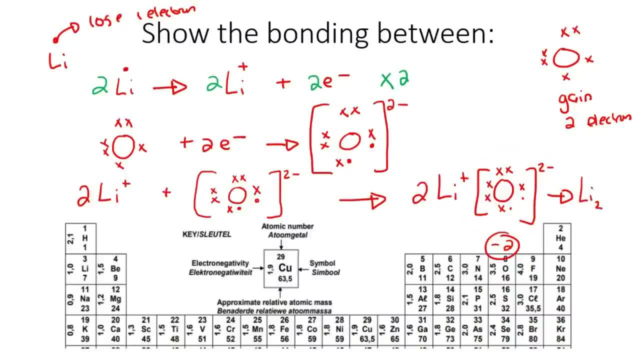 So you'll say Li with a two, And then we have one oxygen like that, And then they might even say that that is a solid. Let's do another example, even more challenging example. Now we're going to do aluminium And we are going to do oxygen. 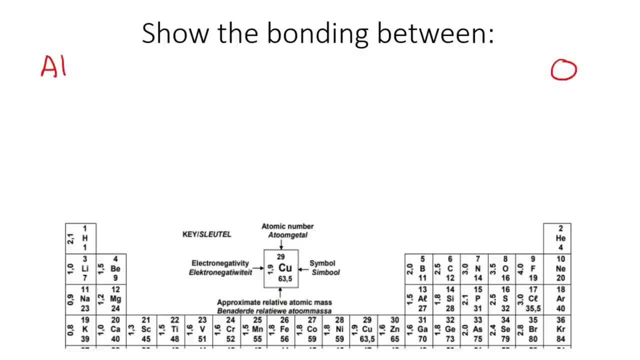 Okay, This is the most challenging example you can get with ionic bonding. So if we look at the Lewis diagram of aluminium, we can see that it is in group one, two, three. So it's in group three, Okay. So if we look at oxygen, it's in group six. 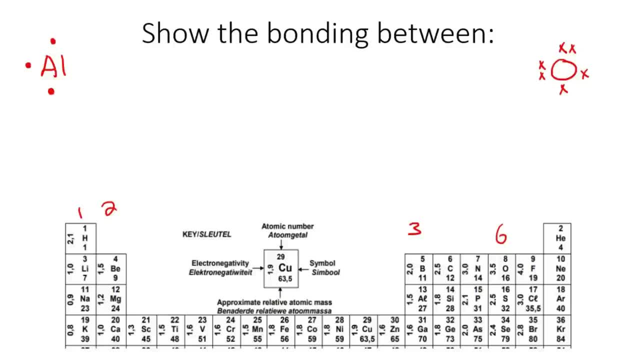 So we put six valence electrons. Okay, Now we know that this aluminium is going to lose three electrons- Remember, we've spoken about that in the past- It wouldn't make sense for it to try gain five things. That would be too difficult. 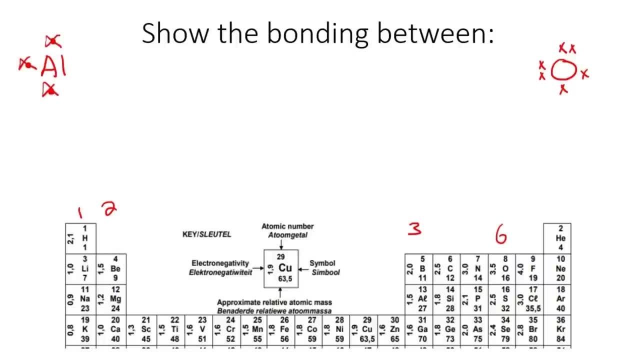 It would rather lose these three. It's rather going to lose those three because it's a metal. It loses electrons. So this is going to lose three electrons. Now this oxygen over here is going to accept two electrons, because then it would be complete. 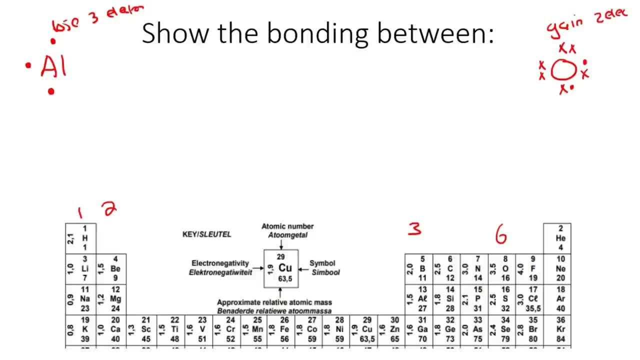 So this one's going to gain two electrons. So whenever you have a metal and a nonmetal, or something that loses with something that gains, that is ionic bonding. Ionic bonding- In later lessons we're going to look at different types of bonding like covalent and metallic. 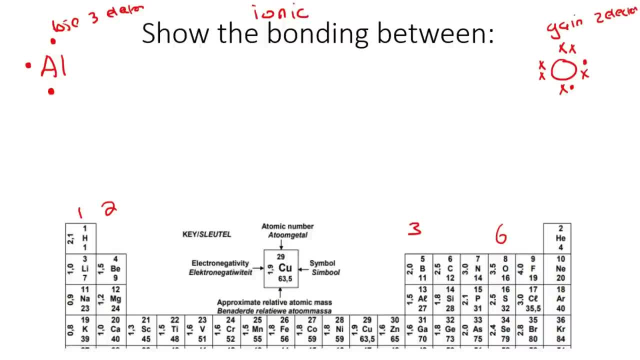 And those are totally different to what we are doing now. So the first step is: let's show that the metal loses its electrons, So it's going to become Al with. all of its electrons are going to be gone. So we're going to say plus three electrons. 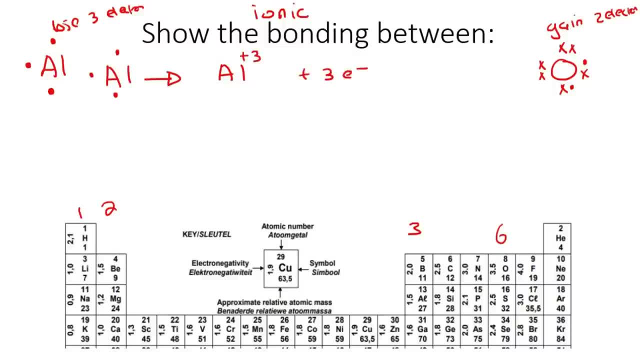 And then, because it's lost three electrons, it's going to become positively charged by three. Okay, And that's the same as its valency. Now, the oxygen is now going to. the oxygen needs to gain two electrons, Okay, And so it would become like that: 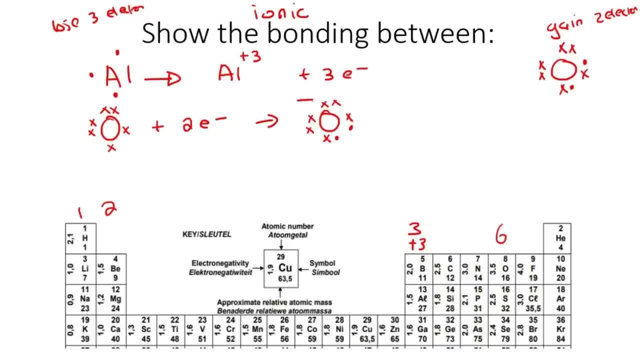 And because it gains two electrons, it becomes negatively charged, So we show it like that. Okay, Now these two numbers are not the same, So we need to make them the same. So what we'll do is we'll multiply this reaction by two. 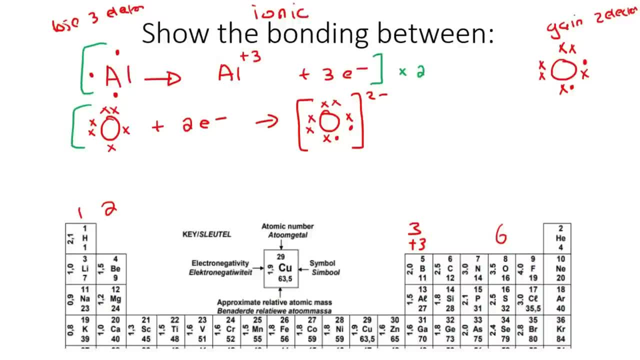 And then we'll multiply this reaction by three. So that means we're going to put a two in the front here, a two in the front here, And this will become a six. Okay, And then we'll put a three in the front here.